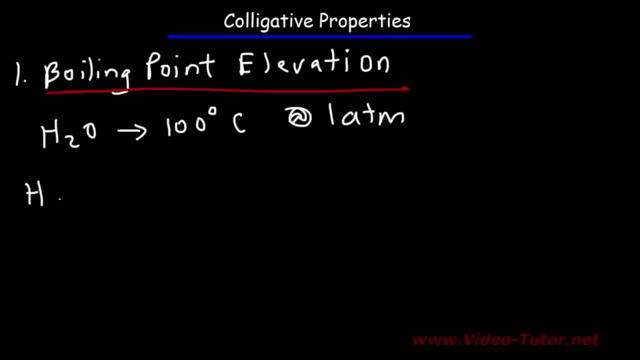 degrees Celsius. Now what happens if we add salt to water? As you add salt to water, the solute water is the solvent, but combined they make up the solution. Now, just to give you some numbers here. this is going to be the molality of the solution and this is going to be the 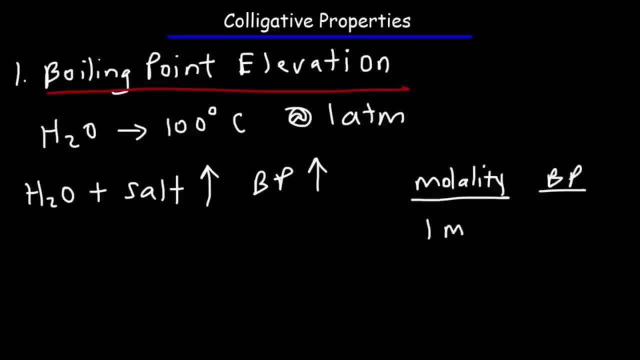 boiling point If you use a one-molo NaCl solution. if you have that, the boiling point is going to be approximately 101 degrees Celsius. If you have a 5m NaCl solution, you're going to have a boiling point of approximately 105 degrees Celsius. Technically it's like 105.5.. And if you 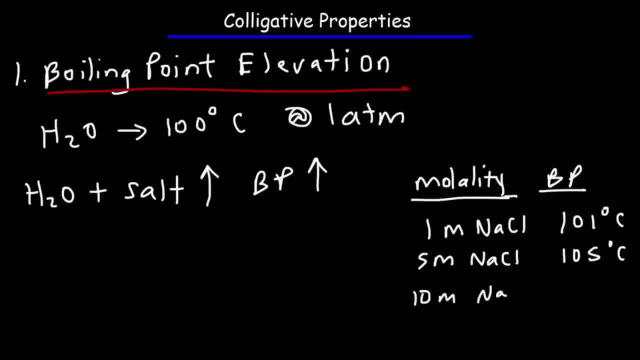 use a 10m NaCl solution. the boiling point is going to be 110 degrees Celsius. To calculate the boiling point, you could use this formula: The change in temperature is equal to Kb times m times I. Kb is the boiling point, elevation constant. m is the molality, I is the Van't Hoff factor. 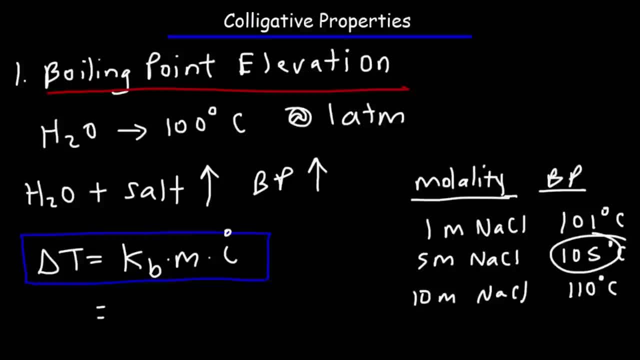 By the way, I think I said 105.5 for a 5m solution. It should be like 105.1.. The Kb for water is 0.51. And if the molality is 5, and the Van't Hoff factor is 2,. 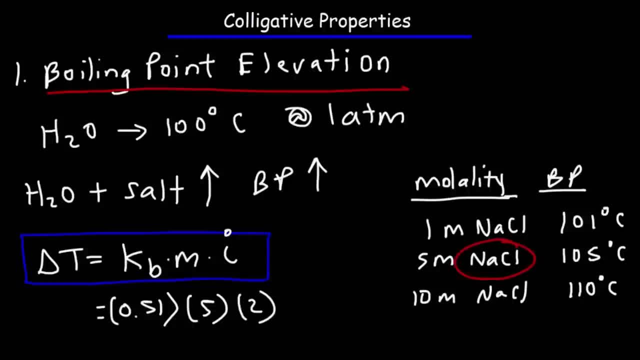 the reason why the Van't Hoff factor is 2 is because when sodium chloride dissolves, the solution is going to be 105.5.. When sodium chloride dissolves in water, it creates two solute particles: Na plus and Cl minus. 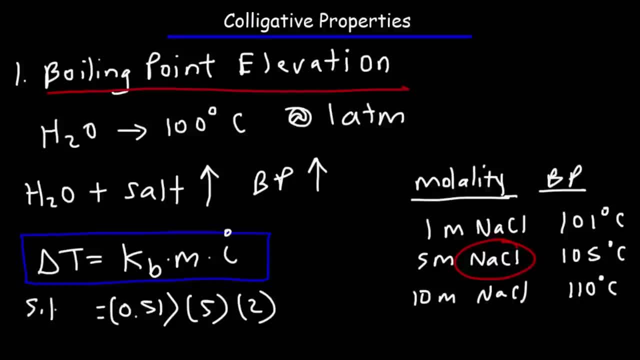 So when you multiply these three numbers out, you're going to get 5.1. That's the change in temperature. So the original boiling point was 100.. Thus the boiling point is going to increase by 5.1. So it's going to be 105.1.. So thus you can see why boiling point elevation is a. 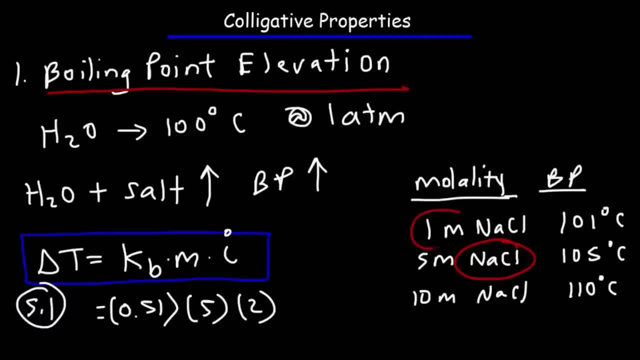 colligative property. It depends on the concentration of the solute particles. As the concentration of the solute particles go up, the boiling point of the solution goes up, And also it depends on the Van't Hoff factor as well, The more ions that are dissolved in. 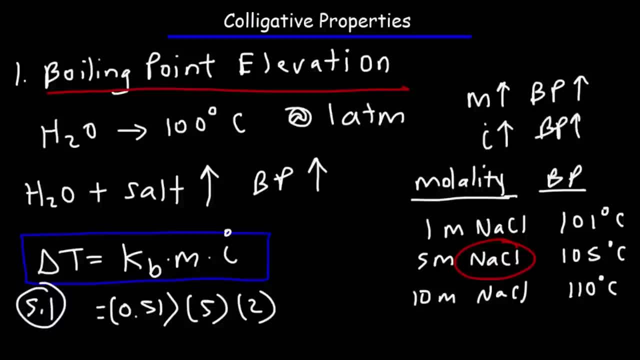 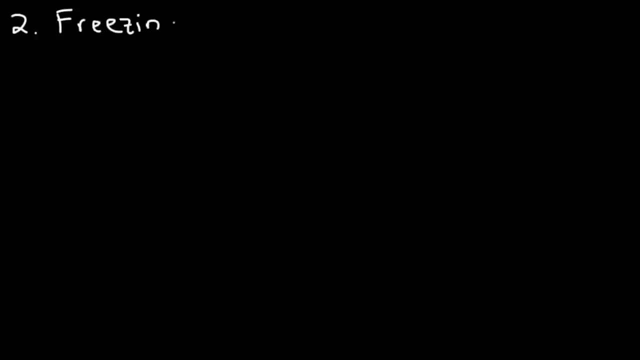 a solution, the boiling point will go up as well. Now, the next type of colligative property that you need to be familiar with is something known as Friesen point depression. So think about what this expression tells you. The word depression means. 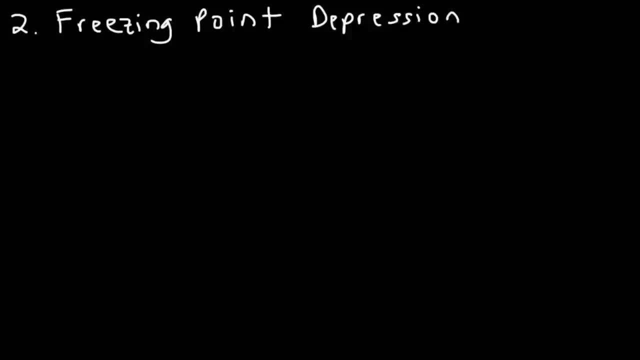 something low, something that's down. So as you add salt to water, the Friesen point, it goes down, it decreases The formula for the Friesen point, depression, it's equal to negative Kf times, the molality times, the Van't Hoff factor, The negative sign is to help you to see that the 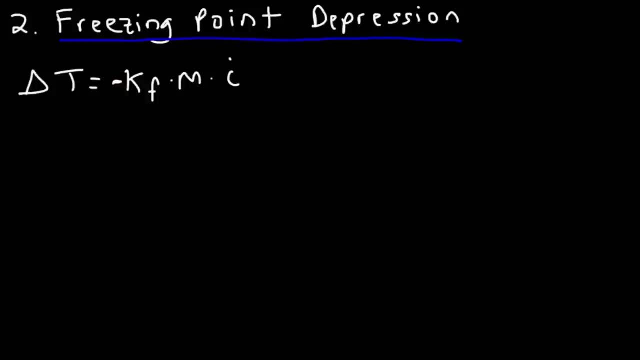 Friesen point goes down: If you don't use the negative sign, then Kf is going to have a negative value. So if you have a positive sign, Kf will be negative. In the case of water it's going to be negative 1.86 degrees Celsius per molality. By the way, molality is equal to 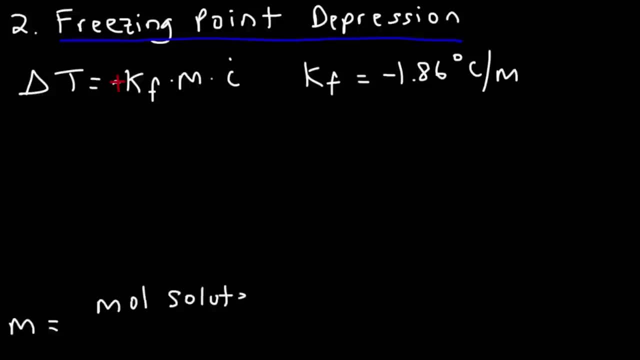 the moles of the solute particles divided by the kilograms of solvent. So that's how you calculate the molality of the solution. for those of you who might be wondering, So as more salt is added to water, the Friesen point- let's put Fp for Friesen point, it goes down. 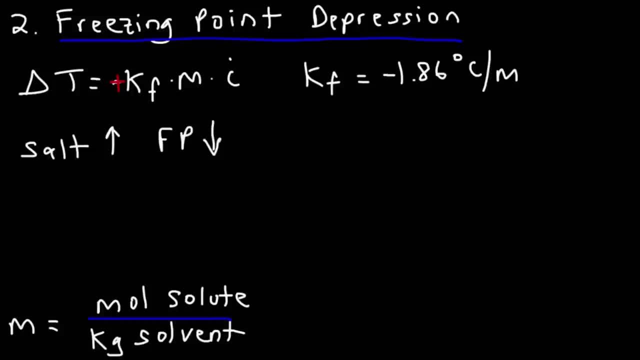 And this property is very useful, particularly in the wintertime. Perhaps, let's say, for those of you who live up north, you probably noticed that during the wintertime, salt is added to the roads in order to prevent Friesen, And when you add salt to water, it makes it difficult for the 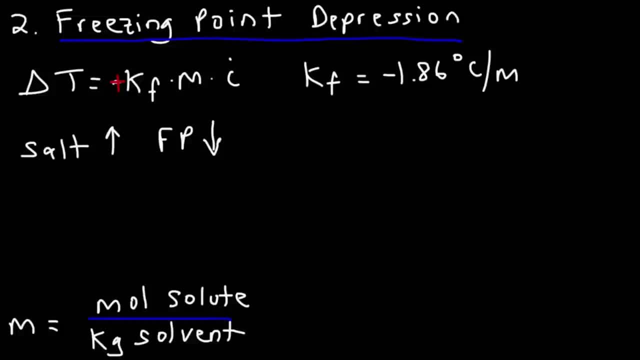 liquid water molecules to freeze, And so that's why adding salt to ice, it helps ice to melt, because the Friesen point goes down, And that's why salt is typically added to the roads in the wintertime. It makes it difficult for ice to form, but easy for ice to melt. Now let's add some. 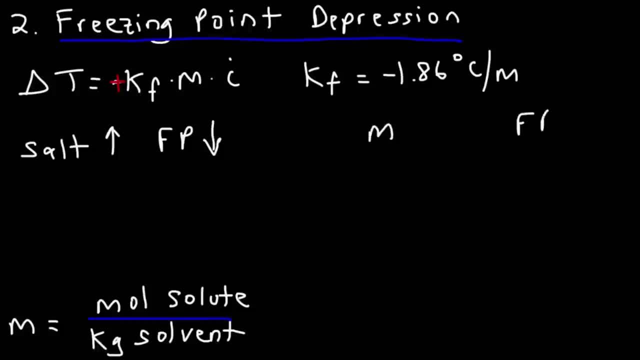 numbers to this situation. So let's see the relationship between molality and Friesen point. If the concentration is zero, then the Friesen point is going to be negative 1.86 degrees Celsius per molality. If the concentration is zero, then the Friesen point is going to be negative 1.86 degrees Celsius per molality. 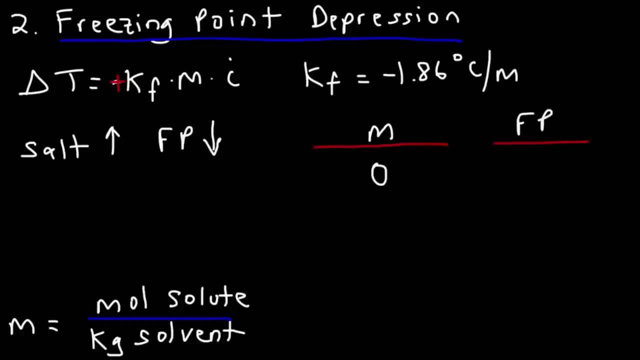 If the concentration is zero, then the Friesen point is going to be negative. 1.86 degrees Celsius per molality. That is the concentration of the solute. We have pure water. Water freezes at zero degrees Celsius. Now if we have a 1m sodium chloride solution, if you multiply negative 1.86 times one, 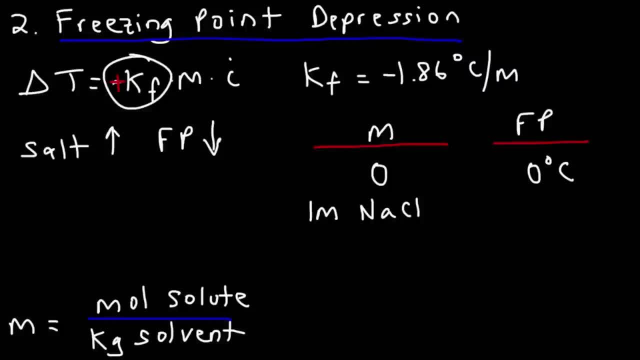 times the two ions in the sodium chloride solution, you're going to get 3.72.. But if you apply the negative sign, it will be negative 3.72.. So that means the Friesen point will decrease by 3.72 degrees Celsius per molality. So that means the Friesen point will decrease by 3.72 degrees Celsius per molality. 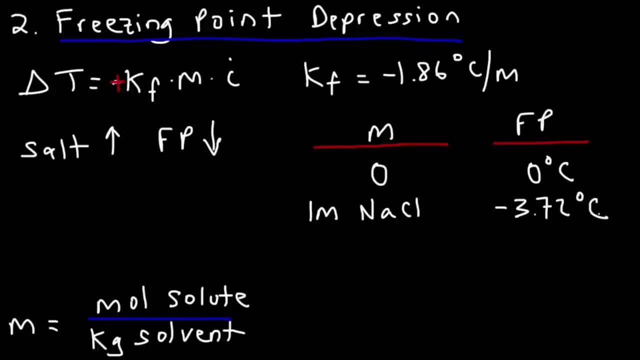 units from zero. So the new Friesen point of the solution will be negative 3.72 degrees Celsius. If we were to increase the solute concentration by a factor of five, the Friesen point will increase by a factor of five. That is the change in a Friesen point. 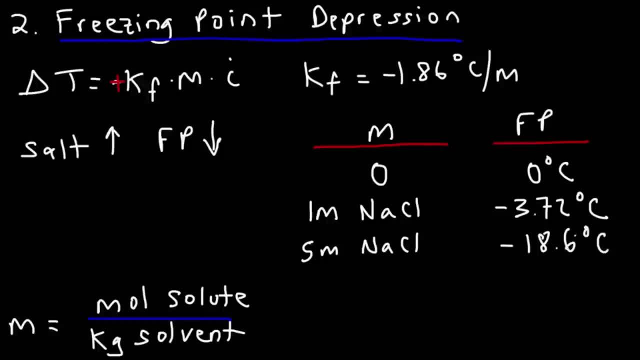 So it's going to be negative 18.6 degrees Celsius. Now let's say if we were to use a 5m solution, but of a different substance, AlCl2.. The identity of the substance doesn't matter, but what matters is the quantity of. 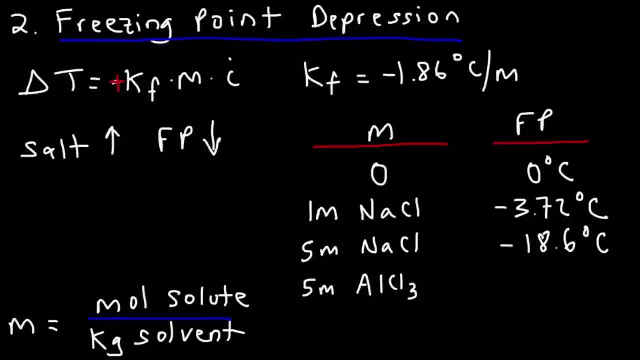 the solute in the substance, AlCl2, can break up into four ions. We can get the aluminium, 3 plus cation, So that's 1 ion, And we can get three chloride ions. So one formula unit generates 4 ions, which means our I value is 4.. 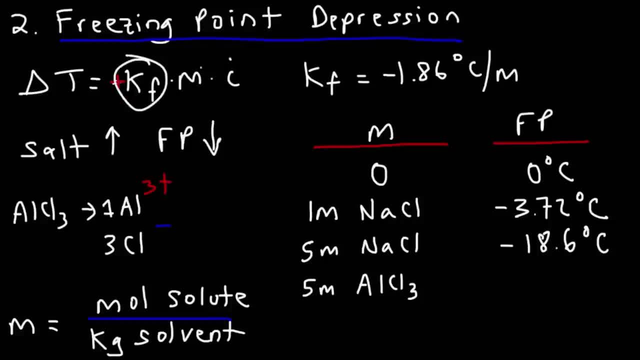 so if you multiply negative one times 3.72 degrees Celsius, 1.86 times 5 times 4, that will give you a freezing point or the change in freezing point, which will be negative: 37.2 degrees Celsius. 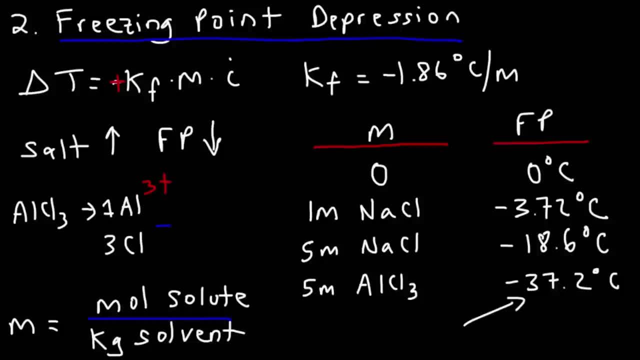 But starting from zero, the new freezing point will be that value. So now you can see why freezing point depression is a colligative property, Because this property depends on the concentration of solid particles. As the concentration goes up, the freezing point depresses, it goes down. 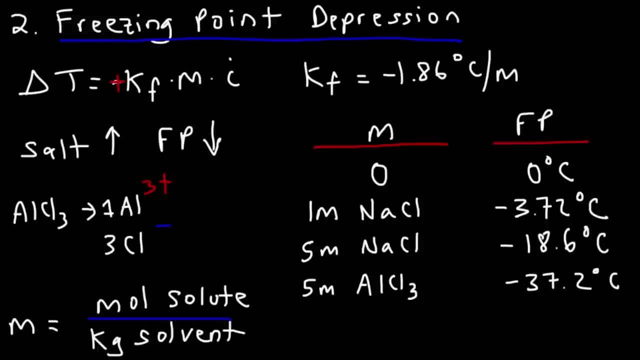 It doesn't depend on the identity of the solid particles, but it depends on the concentration. For instance, if I were to use a 1m solution of Ki, both of these have two ions per formal unit. The identity is different, but the concentration is the same. 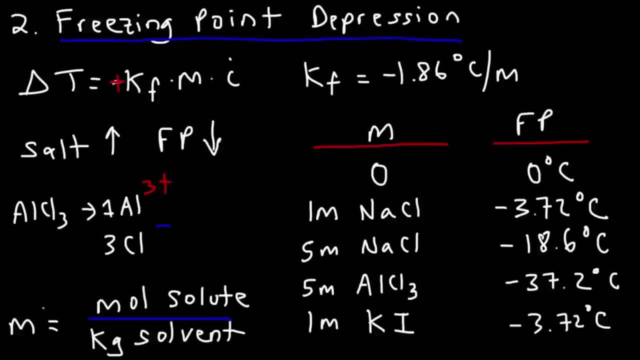 Thus the freezing point will be the same, And that's what makes it a colligative property: It depends on the concentration of the solid particles and not the identity of the solid particles. Now let's move on to the next colligative property. 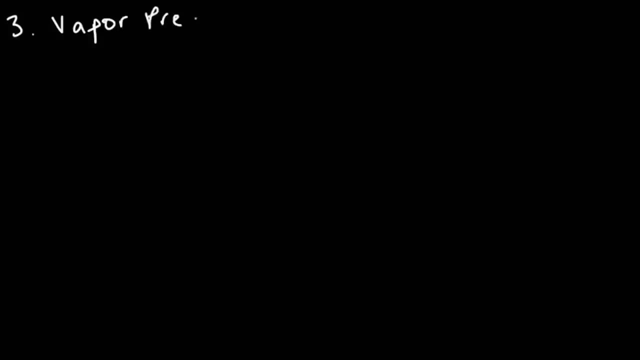 The next one is vapor pressure. This property also depends on the concentration of the solid particles. Now let's briefly talk about why. The vapor pressure of the solution is equal to the mole fraction of the solvent multiplied by the vapor pressure of the solvent. 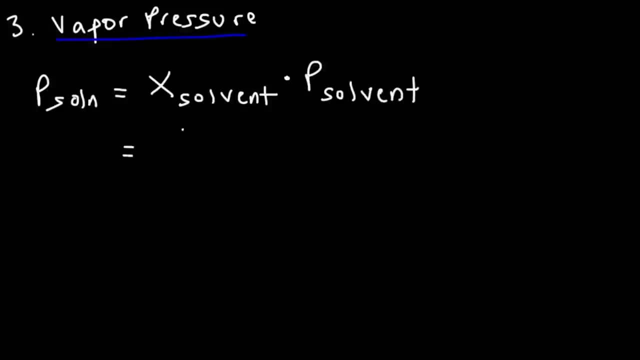 Now the mole fraction of the solvent. let's say, if we're using a salt water solution, the water is going to be the solvent. So this is going to be the moles of H2O divided by the total moles of the solution. 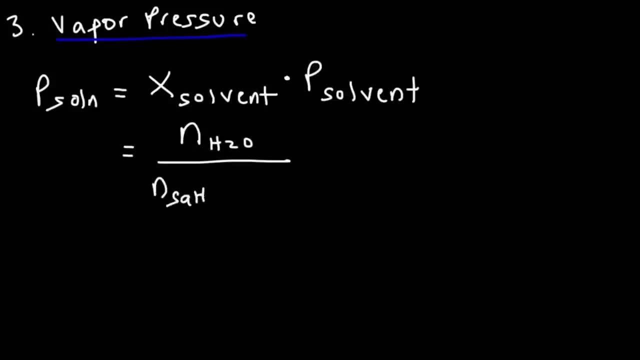 which will be the moles of the salt that we have. let's use sodium chloride plus the moles of water. So, looking at this equation, we could see that the vapor pressure of the solution depends on the moles of solute particles. 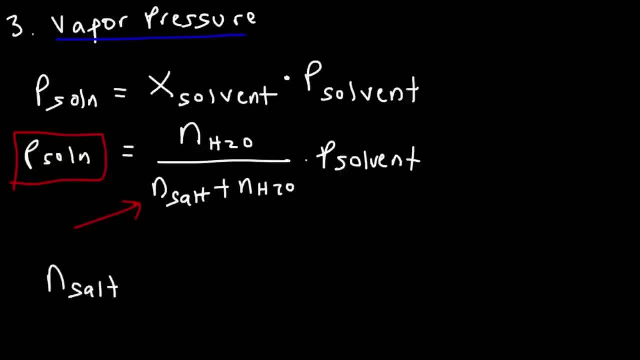 So if we were to increase the moles of the solute particles, what's going to happen to the vapor pressure? Will it go up or will it go down? Well, as we increase the moles of solute particles, we are increasing the value of the denominator of the fraction. 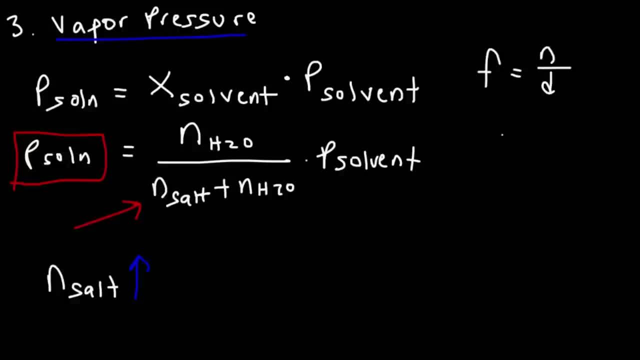 A fraction has a numerator and it has a denominator. Whenever you increase the value of the denominator of a fraction, the value of the whole fraction goes down. There's an inverse relationship between the two. So as we increase the moles of solute particles in the solution, 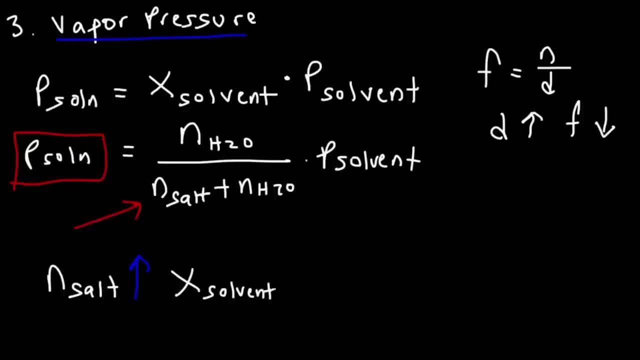 the mole fraction of the solvent, that is, this entire fraction, goes down in value. As the mole fraction of the solvent goes down in value, the vapor pressure of the solution goes down in value, And so we see an inverse relationship between solute concentration and the vapor pressure of the solution. 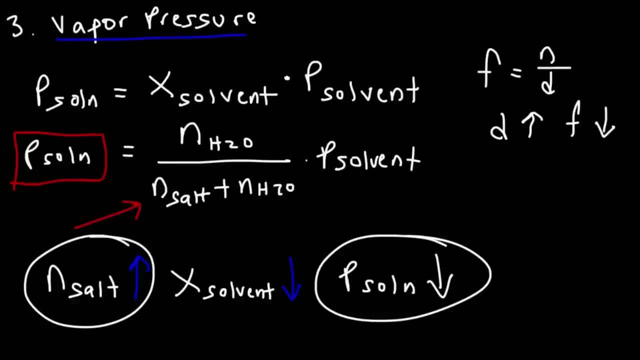 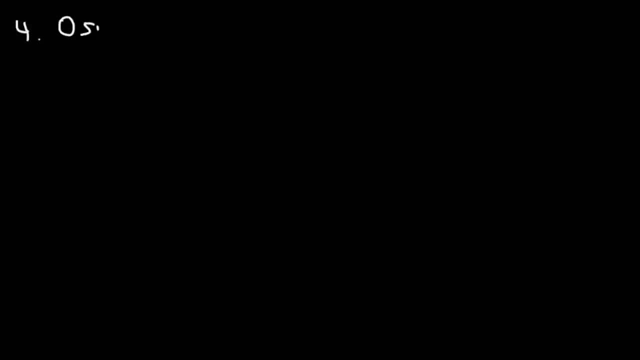 As the moles of the solute goes up, the vapor pressure of the solution goes down, making it a colligative property. Now let's consider the fourth one. The fourth colligative property we're going to talk about today is known as osmotic pressure. 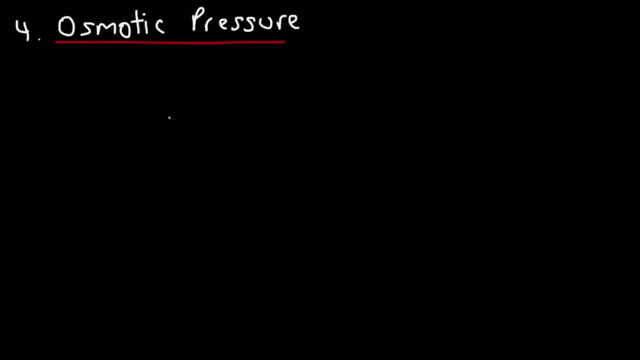 Here's the formula for osmotic pressure: It's pi is equal to MRT times the Van't Hoff factor. I Capital M is the molarity, R is the gas constant, 0.08206, and it's liters times atm divided by moles times kelvin. 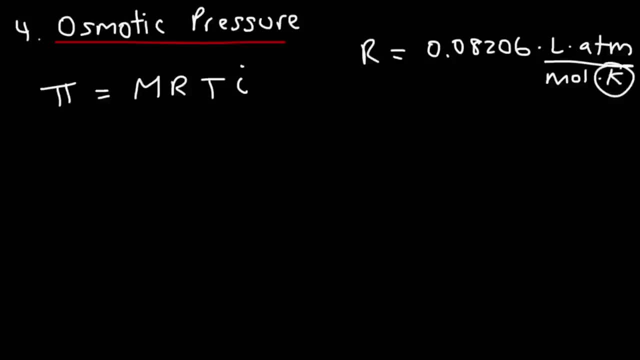 So because R has the units kelvin, the temperature has to be in kelvin. Keep in mind the kelvin temperature is the Celsius temperature plus 273.15.. The molarity is different than molality. Keep in mind. molarity is the moles of solute divided by the liters of solution. 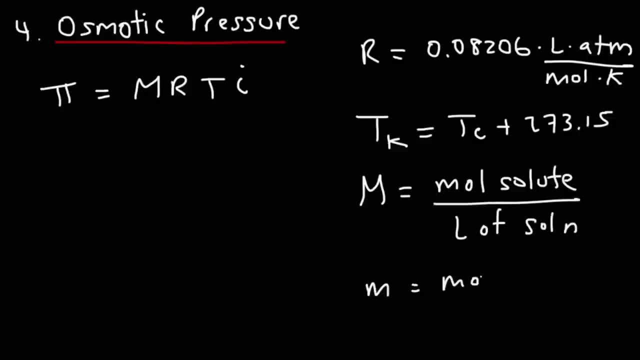 And let's contrast that with molality. Molality is equal to the moles of solute divided by the kilograms of solvent. So both of these quantities, these are different forms of concentration, But the result is the same As we increase the concentration of the solute particles. 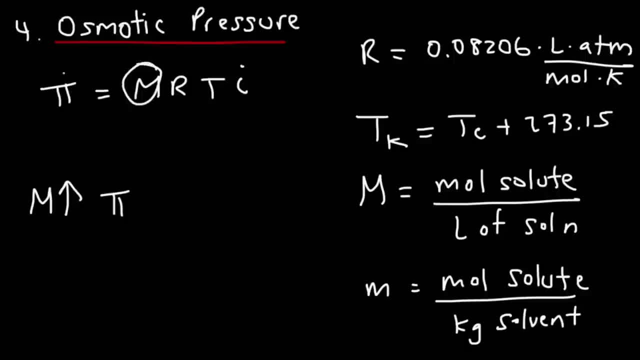 the osmotic pressure is affected. In this case there is a direct relationship between the two. The osmotic pressure goes up. So let's review the four colligative properties. Number one: boiling point elevation As you increase the concentration of the solute particles. 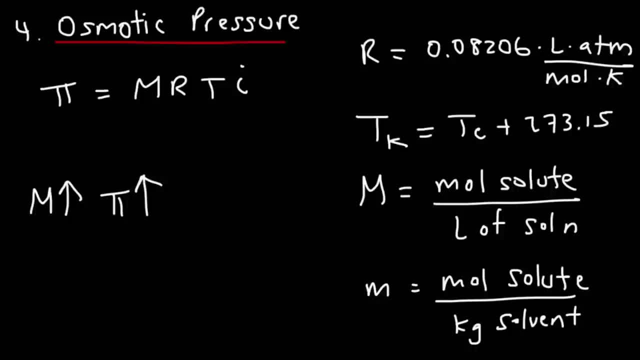 boiling point goes up. Number four: osmotic pressure. As you increase the molarity, osmotic pressure goes up. So for those two there's like a direct relationship. Now for number two and three. freezing point: depression and vapor pressure. 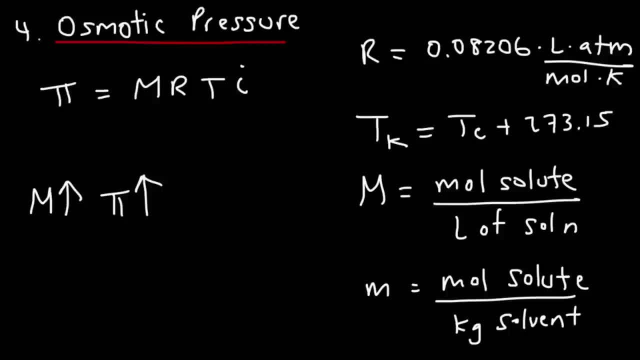 there's like an inverse relationship: If you increase the solute concentration, the freezing point goes down, And if you increase the solute concentration, the vapor pressure goes down. So let's just write that down. Let's just write that so you can see a summary. 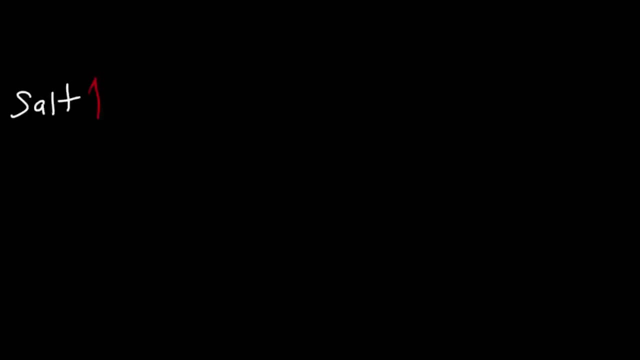 So as we increase the concentration of the solute or the salt, the boiling point goes up and the osmotic pressure goes up, The vapor pressure goes down. and what was the other one, Freezing point, The freezing point. The freezing point goes down as well. 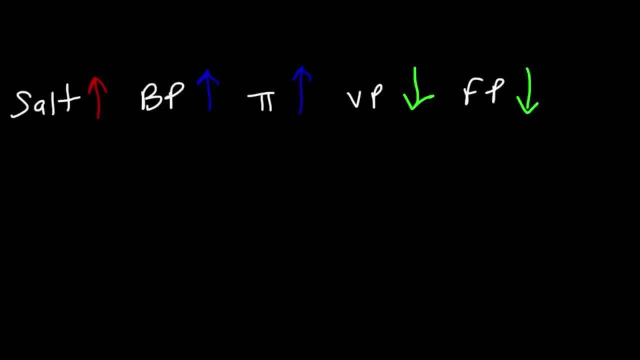 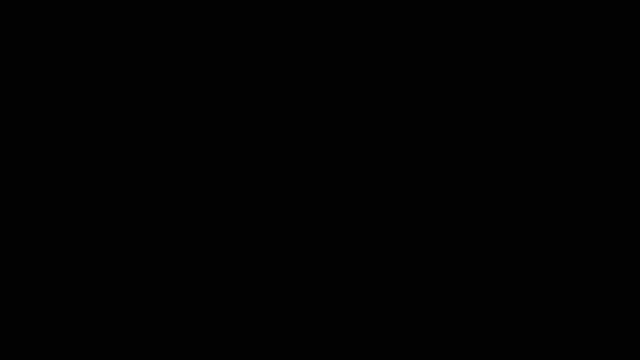 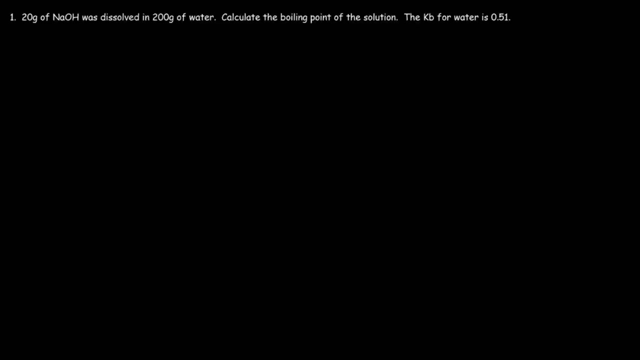 So that's the relationship between the saline concentration and the four colligative properties. Now let's work on a few problems associated with boiling point elevation and freezing point depression. So in this example problem we have 20 grams of sodium hydroxide dissolved in 200 grams of water. 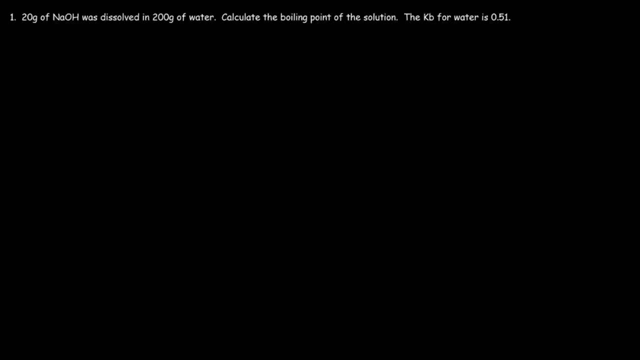 Our goal is to calculate the boiling point of the solution, And we're given the boiling point elevation constant Kb. It's 0.51.. So what can we do here? This is the formula that we need. The change in the boiling point is going to be equal to Kb times the molality of the solution, times the Van't Hoff factor. 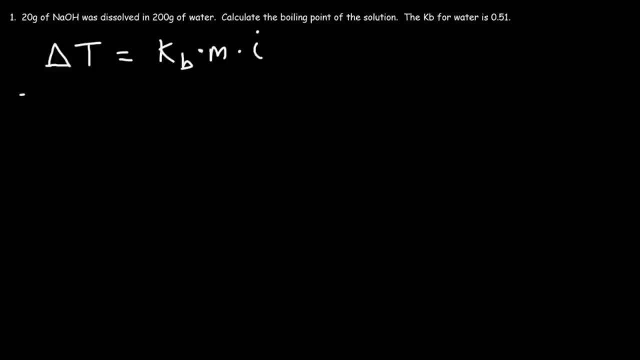 The delta T is the difference between the boiling point of the solution and the saline concentration. This is the difference between the boiling point of the solution and the boiling point of pure water. So I'm going to move this to the other side of the equation. 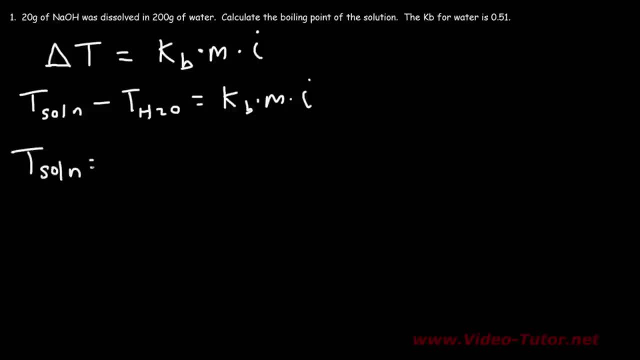 So the boiling point of the solution is going to be the boiling point of pure water plus Kb times M times, Kb Times M times I. So we know the value of Kb. And for the Van't Hoff factor, sodium hydroxide consists of two ions. 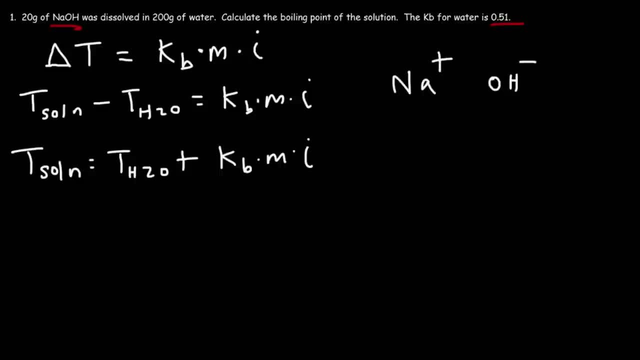 The Na plus ion and the hydroxide ion. So when sodium hydroxide is dissolved, that one formula unit becomes two ions. Thus the Van't Hoff factor is 2 for this problem. Now, the only thing that we're missing is the molality of the solution. 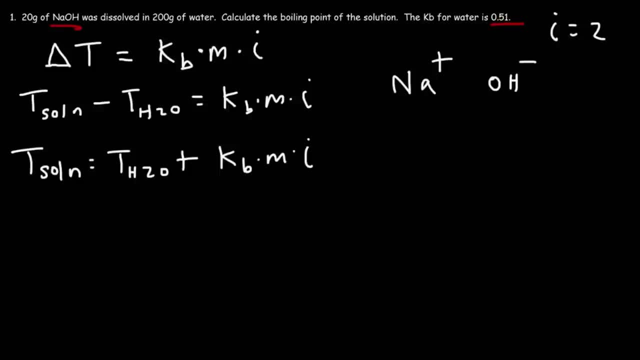 Molality is moles of solute divided by kilograms of solvent. So we're given the grams of the solute- 20 grams of sodium hydroxide. What we need to do is convert it to moles. To do that, we need the molar mass of NaOH. 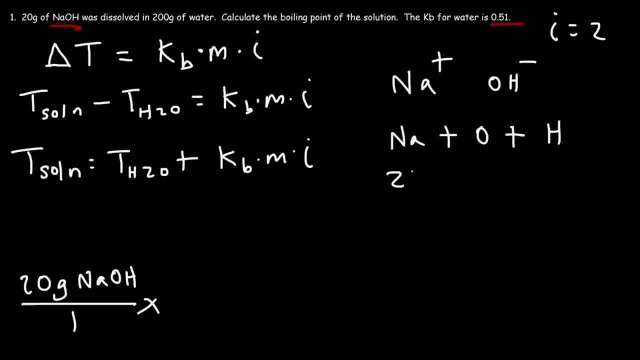 So we need the periodic table. The atomic weight of sodium is 22.99.. Let me get my periodic table Just to make sure I have it correct. And yes, that's it 22.99.. For oxygen it's 16.. 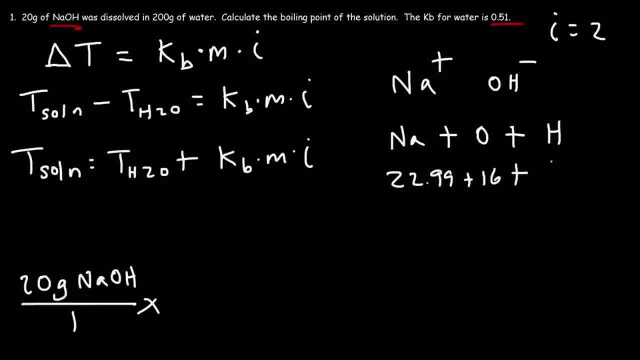 And for hydrogen it's 1.008.. So this is 39.998, which I'm going to round to 40. Because 20 and 40 is like just half of each other. So one mole of sodium hydroxide has a mass of approximately 40 grams of sodium hydroxide. 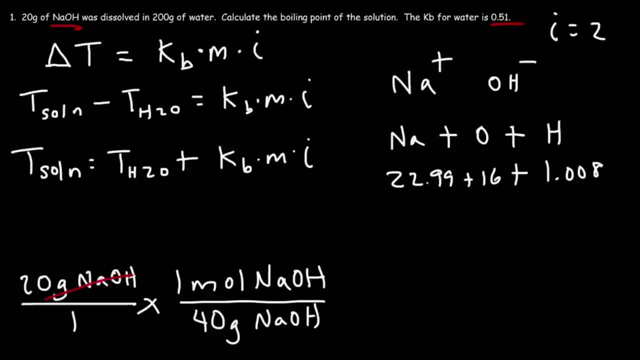 So the unit grams cancel. and now we have moles of solute And we need to divide this by the kilograms of the solvent. The solute is NaOH, the solvent is water, So we need to convert 200 grams to kilograms. 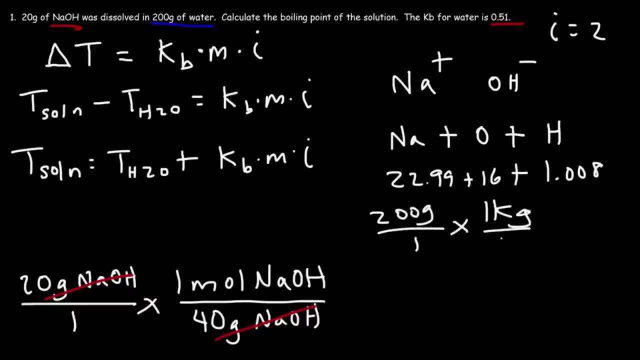 One kilogram is 1,000 grams. So any time you need to convert from grams to kilograms, simply divide by 1,000.. 200 divided by 1,000 is 0.2.. So we're going to divide the moles of solute by 0.2 kilograms of solvent. 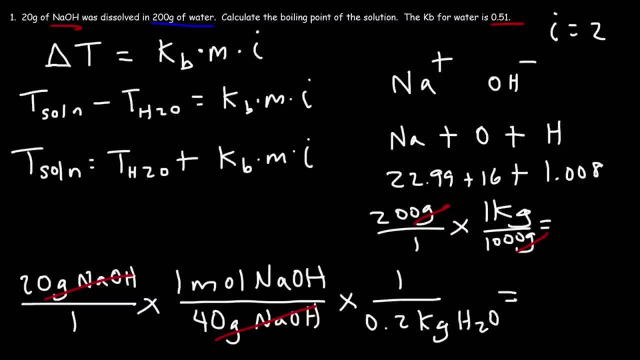 So this here is going to give us the molality of the solution. Now let's get rid of that And let's plug in the numbers. So 20 divided by 40, that's 0.5.. 0.5 divided by 0.2 is 2.5. 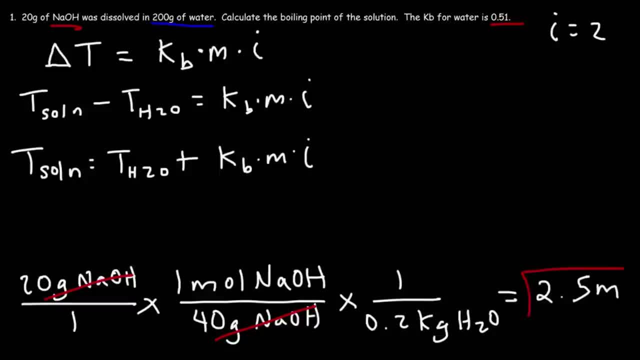 So that is the molality of the solution. Now let's plug in everything into this formula. So we have the boiling point of water, Or at least we know what it is- The boiling point of pure water at atmospheric pressure of 0.2 kilograms. 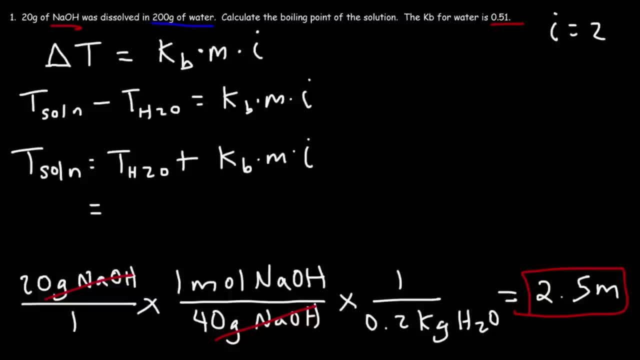 Let's say, at sea level, at an atmospheric pressure of 1 atm, That is 100 degrees Celsius. Now Kb is 0.51, with the units Celsius per molality times a 2.5 molal solution times a Van't Hoff factor of 2.. 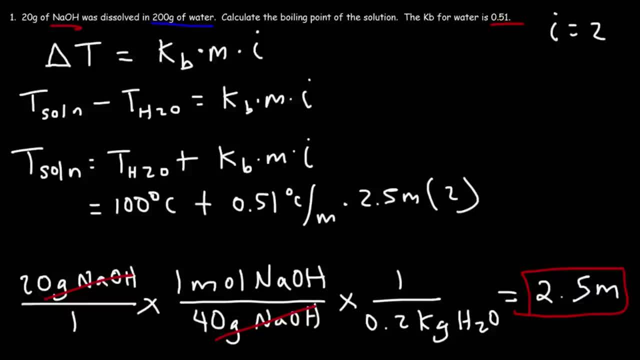 So 0.51 times 2.5 times 2. That's 2.55.. And then, once we add that to 100, we're going to get the boiling point of the solution, Which is 102.55 degrees Celsius. 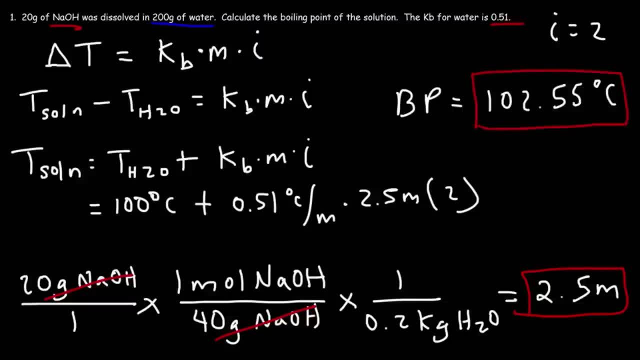 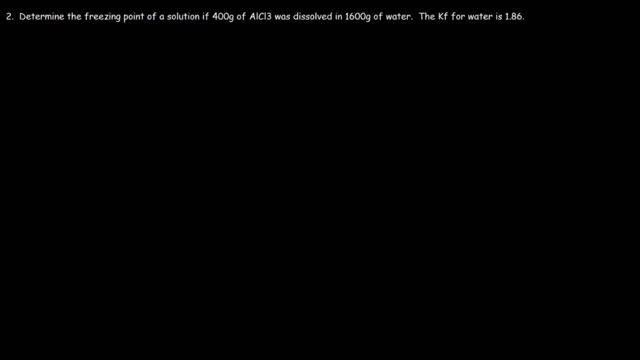 So that's how you can calculate the boiling point of a solution when you dissolve a solute in water. Now let's move on to the next problem, Number 2.. Determine the freezing point of a solution if 400 grams of aluminum chloride 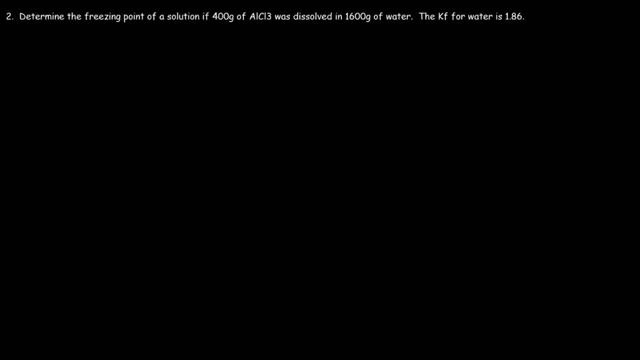 is dissolved in 1600 grams of water And we're given the Kf for water. It's 1.86.. So the boiling point of the solution is going to be the boiling point of the pure solvent, which is water again. 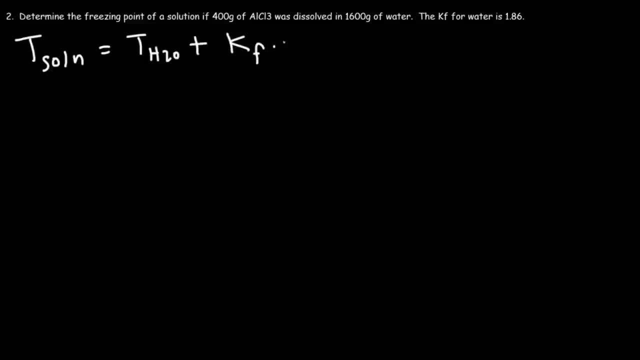 But this time it's going to be plus the Kf value times the molality, times the Van't Hoff factor. Now we're dealing with aluminum chloride. When you dissolve aluminum chloride in water, it's going to break up into the aluminum 3 plus cation. 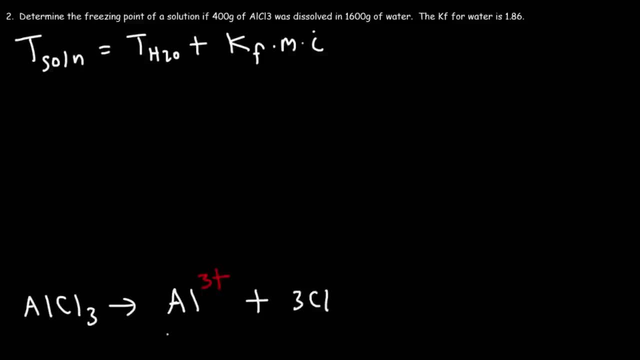 And we're also going to get 3 chloride ions. So notice that we get a total of 4 ions per formula unit. Thus the Van't Hoff factor is going to be 4 in this example. Now let's calculate the molality. 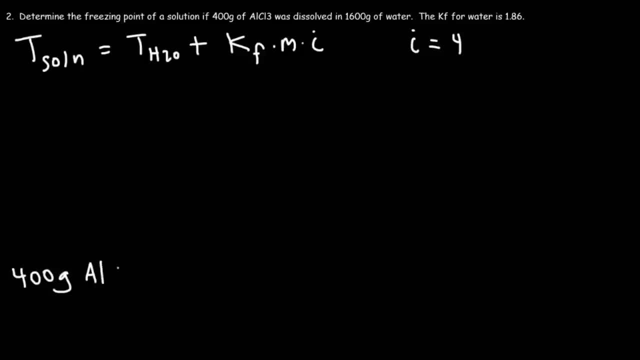 So let's start with the grams of solute, just like we did in the last problem. So we need to convert grams of aluminum chloride into moles, which means we need the molar mass of AlCl3.. So we have 1 aluminum atom. 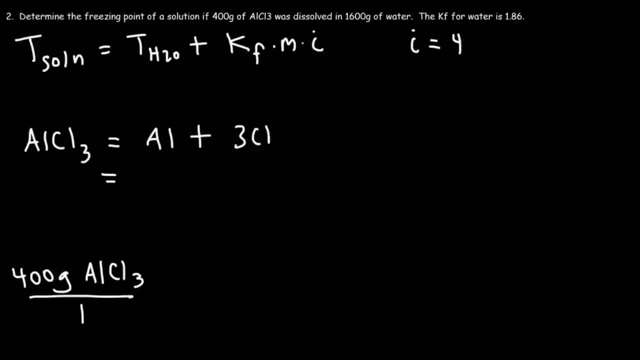 and 3 chlorine atoms. Using the periodic table, the atomic weight of aluminum is 26.98 and the atomic weight of chlorine is 35.45 times 3.. So let's perform the computation. So this gives us a molar mass of 133.33. 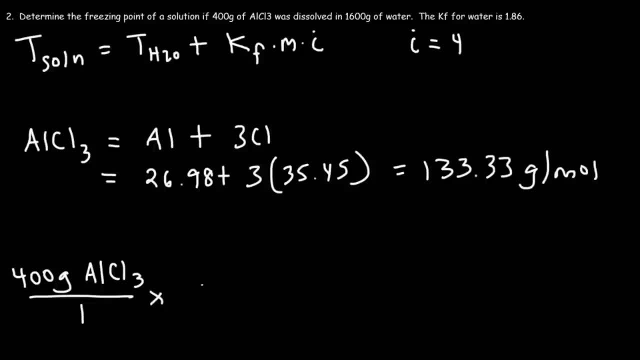 grams per mole. So this tells us that 1 mole of AlCl3 equates to a mass of 133.33 grams. Now our next step is to divide the moles of solute by the kilograms of solvent. So we have 1600 grams of water. 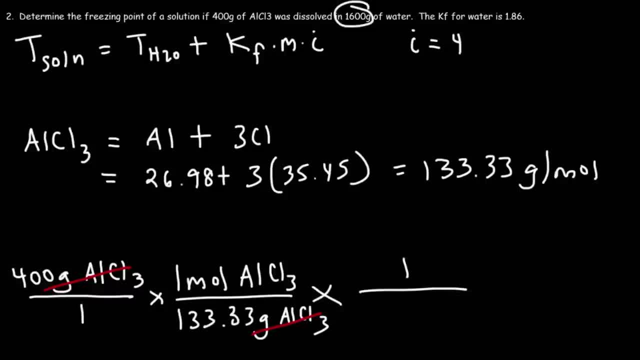 If we divide 1600 by 1000, it's going to give us 1.6 kilograms of solvent. So remember, the molality is equal to the moles of solute divided by the kilograms of the solvent. So this is going to be 400. 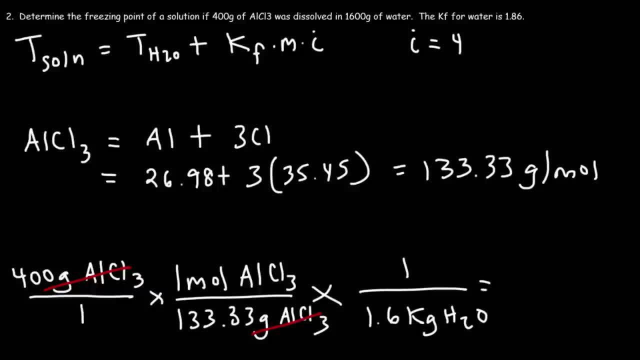 divided by 133.33, which is essentially 3, and 3 divided by 1.6 gives us this answer: 1.8 solute. So that's the molality of the solution. Now let's plug in everything to get the final answer. 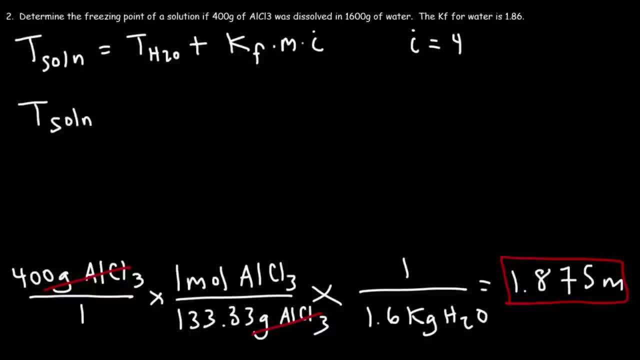 So the boiling point- I mean rather the freezing point of the solution- is going to be the freezing point of water, which is 0 degrees Celsius plus Kf. Now, whenever you add a solute to water, the freezing point goes down. This is freezing point depression. 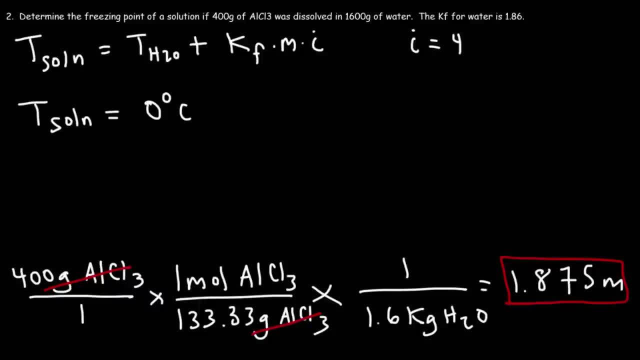 When you add a solute to water, the boiling point goes up, Thus the expression boiling point elevation. So in this problem the Kf for water is going to be negative because it depresses or decreases the freezing point. So this is going to be negative. 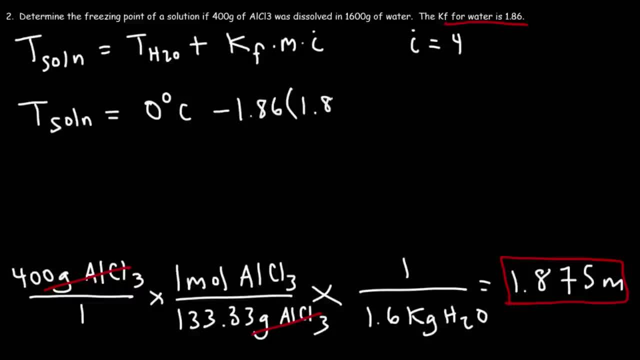 1.86 times a molality of 1.875 times the Van't Hoff factor of 4.. And so we're going to get negative 13.95 degrees Celsius. So that is the freezing point of the solution. Now let's. 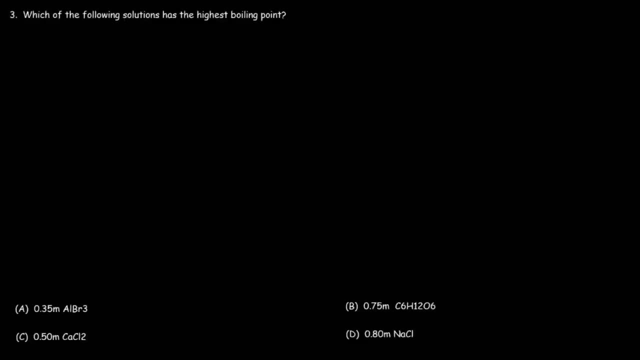 move on to the last problem in this video. Which of the following solutions has the highest boiling point? Is it A, B, C or D? Well, let's write the equation. We know that the change in temperature is going to be equal. 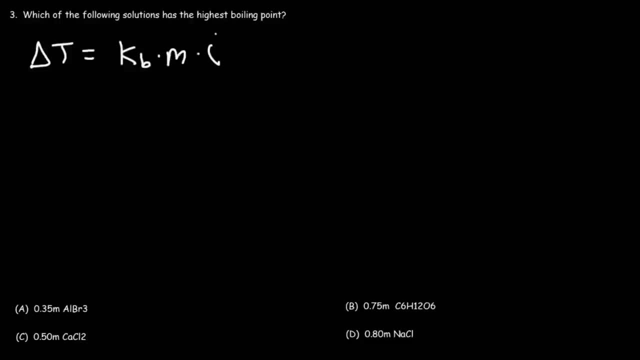 to Kb times M times I. Now Kb is going to be constant for all of the solutions. We're assuming that the solvent is the same, most likely water. So the only part that's different is the Mi product, Because for each of the four